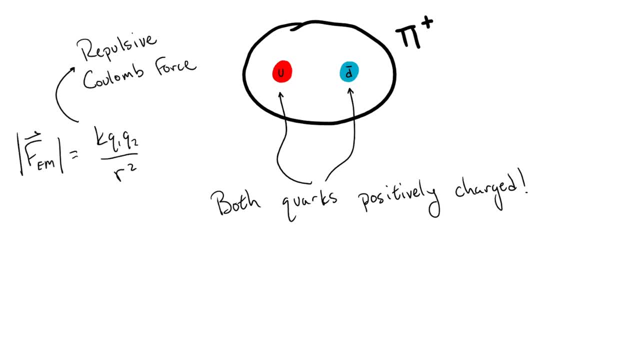 to be bound together. But if this is the case, how is the massive electromagnetic repulsion overcome in order for these bound states to form? Another question, which was astutely pointed out in the comments of the previous video, has to do with the hadrons. 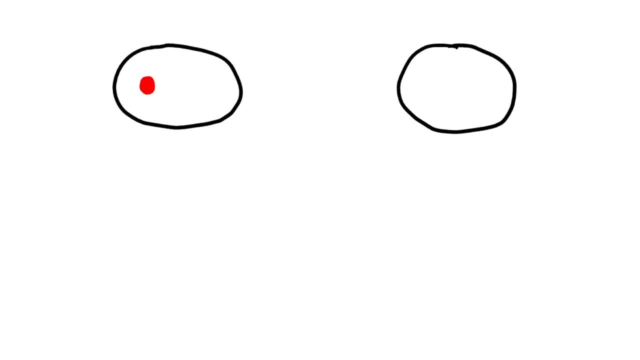 In particular, we discussed, using arguments about electric charges of the mesons, that these states must be made up of quark-anti-quark pairs. Just based on isospin arguments, though, meson states like a combination of one up quark and one down quark should be possible, but these aren't. 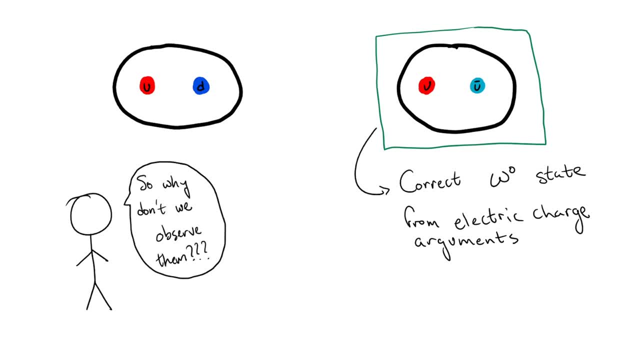 observed. So what disallows these states from existing in nature? These are both fantastic questions which we would like to answer in the comments below. If you have any questions, we will address, but our starting point will be a little more subtle. In particular, we will look. 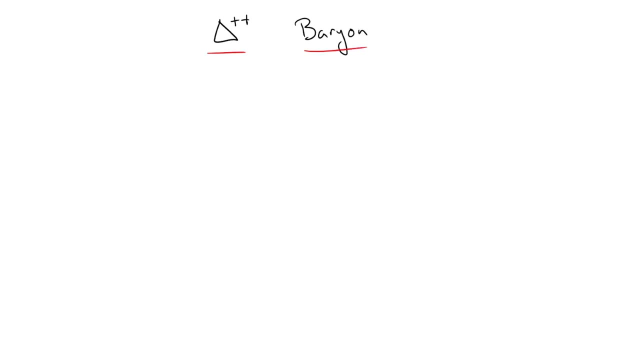 at the delta plus plus baryon, though the same arguments apply to the delta minus as well. This unassuming particle, when considered in more detail, seems to raise some big issues with the quark model. We know from isospin arguments that this particle is made up of. 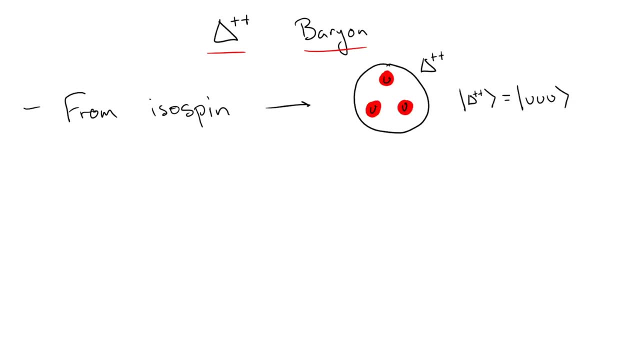 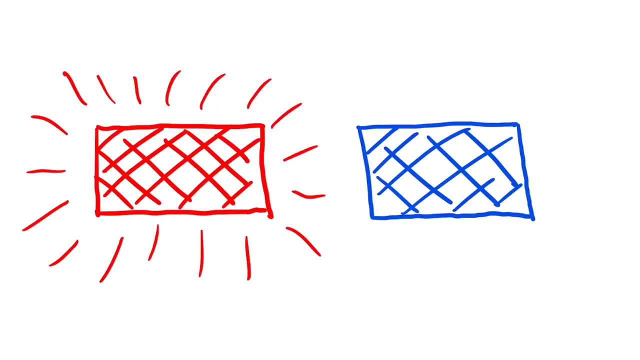 three up quarks. It's also a total spin three halves particle, which means that it can be in a plus three halves state, In which case all three up quarks in the delta plus plus would need to be in the spin up state. This should raise major red flags. We're trying to say that this. 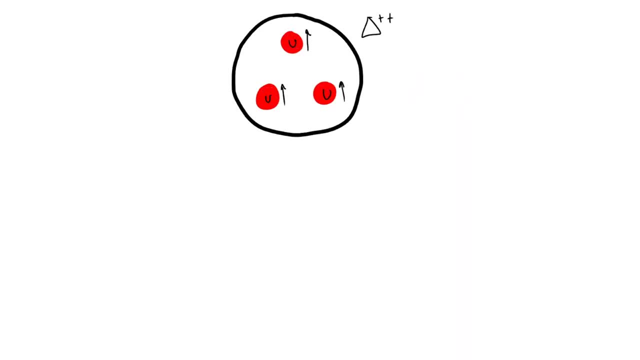 baryon is made up of three identical fermions all up quarks in the spin up state. But this is completely forbidden by the Pauli exclusion principle. We can never have more than one fermion in the same quantum state. So if we're going to do this, we're going to have to. 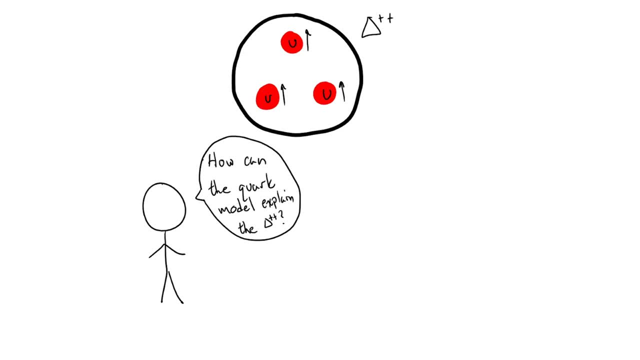 measure the delta plus plus baryons in nature. How can they possibly be explained by this quark model? Well, as it turns out, there is a simple answer. Just require that the three quarks are in fact in different states. This means that we need to give the quarks an extra quantum number. 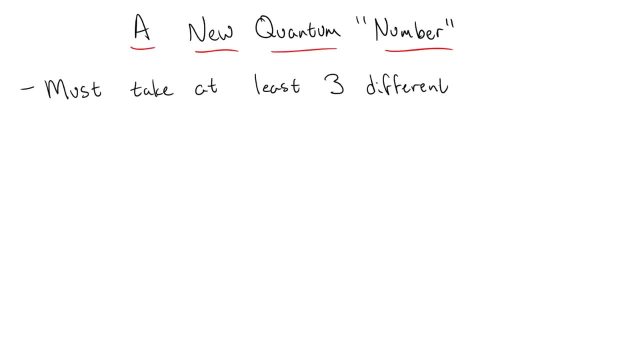 that takes at least three values, so that the three quarks in the delta plus plus can have different values of this quantum number and thus are not identical. Let's again assume that nature prefers simplicity and choose the minimal case where this number can. 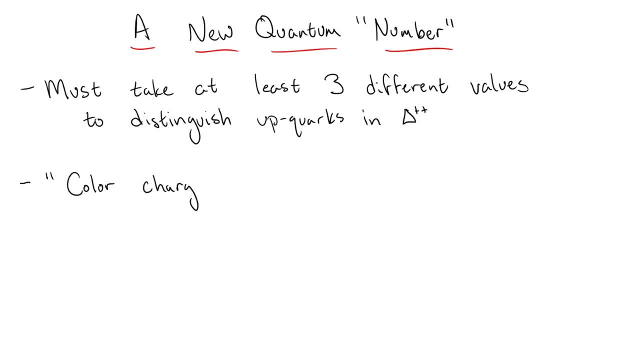 only take three values. Traditionally, this quantum number is known as color charge and its possible values are red, green and blue, but a general state can be constructed from any linear combination of these colors And as long as the color states of the three quarks in the 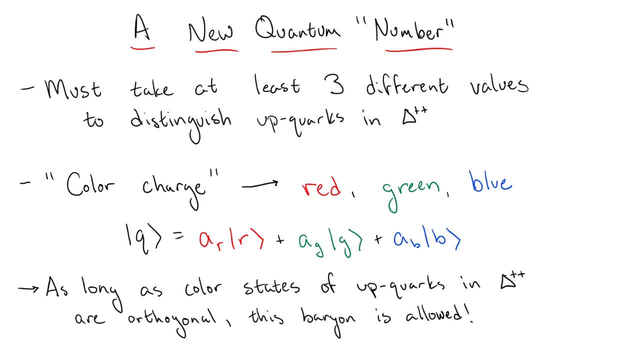 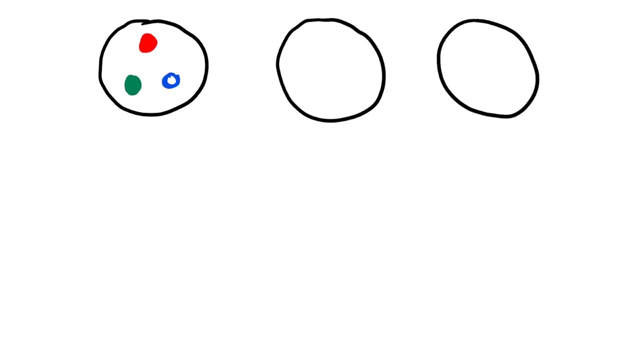 delta plus plus are orthogonal, this baryon is perfectly allowed. This last statement is interesting. We can form this delta plus plus baryon- and any other baryon for that matter- from a bound state of three quarks, each of which. 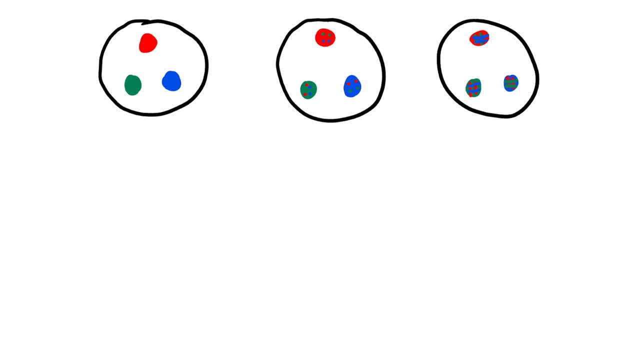 is in an arbitrary color state, as long as all three are orthogonal. If they are not orthogonal, then pieces of the fermionic state are the same and thus not allowed by the Pauli exclusion principle. If this is the case, we might expect to find a continuous spectrum of each type of baryon. 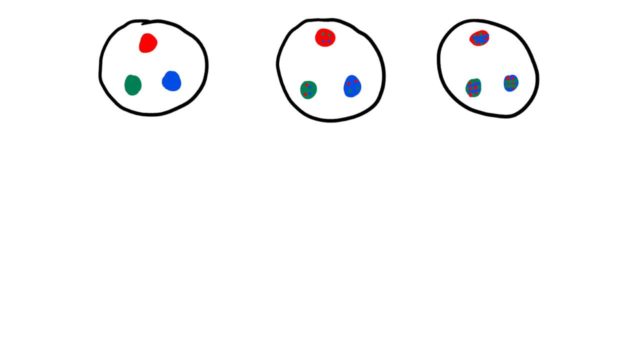 Each piece of the spectrum corresponding to a different set of states of the internal quarks. However, this isn't what we observe. We don't even see a discrete spectrum, like we do with the different spin states of each particle. This means that an arbitrary change to the color states of 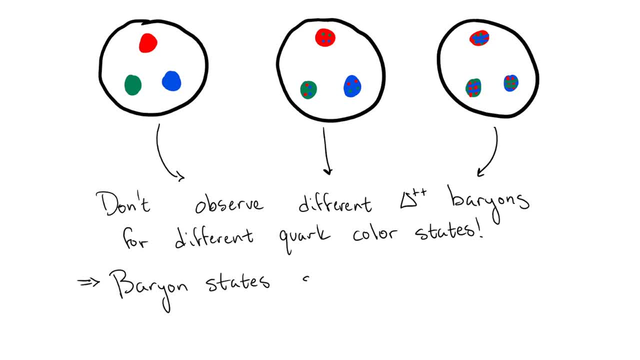 the quarks, keeping the states orthogonal, will always correspond to the same baryon. In other words, the baryons are symmetric under transformation and the quarks and antiquarks in the mesons should carry color charge. but we still don't see. 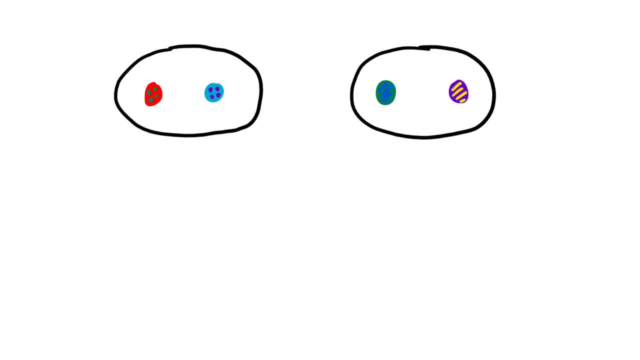 different mesons corresponding to different quark colors, so these states must also be symmetric under these color transformations. What exactly do these color transformations look like? Well, as we have discussed previously, fermions like the quarks are mathematically described by: 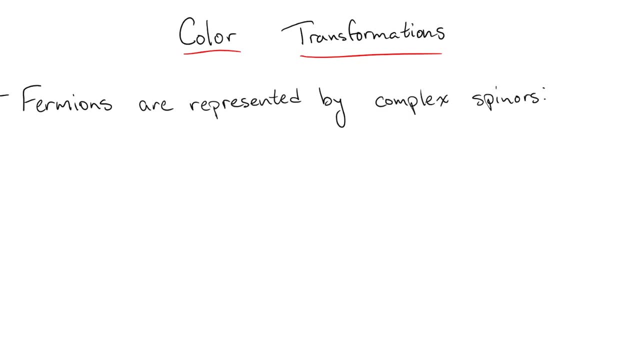 common transformations of the mesons. For example, in the case of the baryon, the fermions are complex spinors, which means that we can think of the color state of a quark as a vector in some internal three complex dimensional space. Then transformations just correspond to rotations. 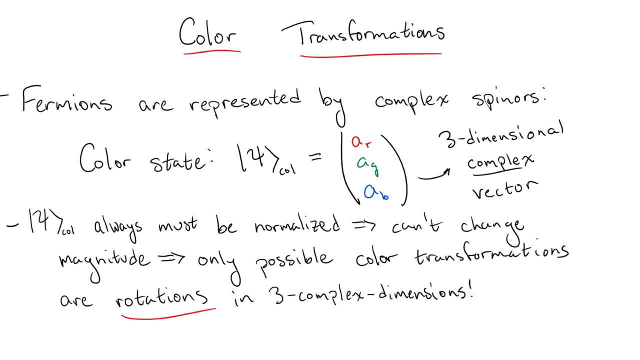 in this internal space. Notice that this is very reminiscent of what we saw when considering QED, where the theory was symmetric under rotations in an internal complex plane. The collection of these three complex dimensional rotations actually has a special name in mathematics, known as SU3.. The SU stands for special unitary. 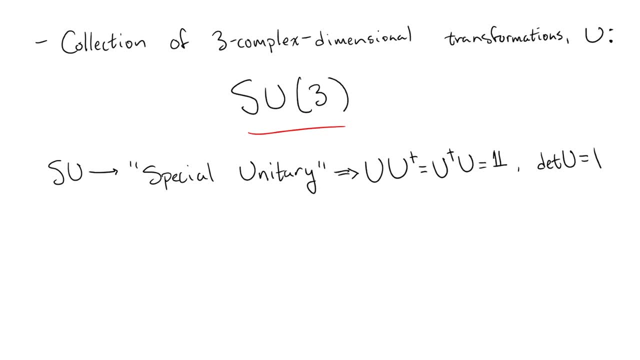 and just tells us certain properties of the transformations which are allowed, namely that the conjugates of the transformations are their inverses and that they have unit determinant. The 3 tells us that the simplest space that these transformations act on is three-dimensional, the complex part being implied by the unitarity of the 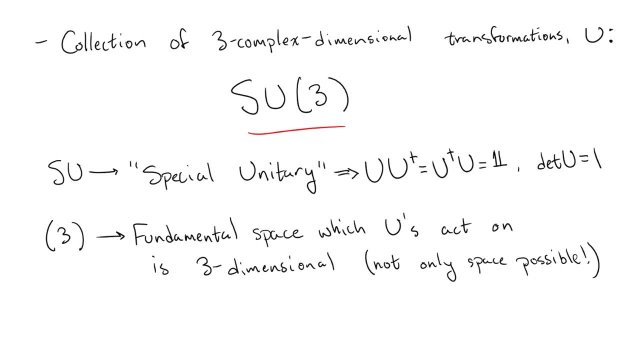 transformations. Note that this naming convention applies to QED as well, whose transformations are part of the U1 group. The S is left off here, since all U1 transformations automatically have determinant 1.. Now these SU3 transformations don't have to only act on three-dimensional complex objects. 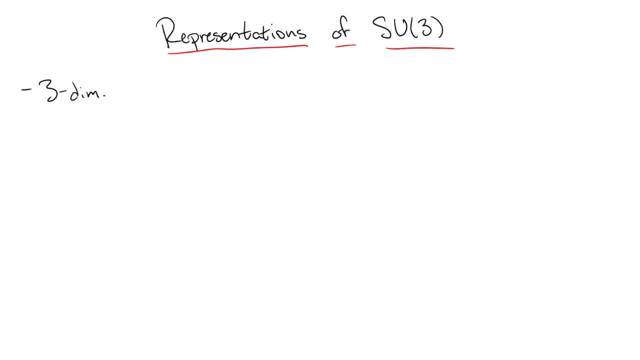 Specifically, we say that these three-dimensional objects furnish the fundamental representation of SU3.. However, there are other representations of these transformations, such as the U1 group, For example. there is an anti-fundamental representation of SU3, which can be. 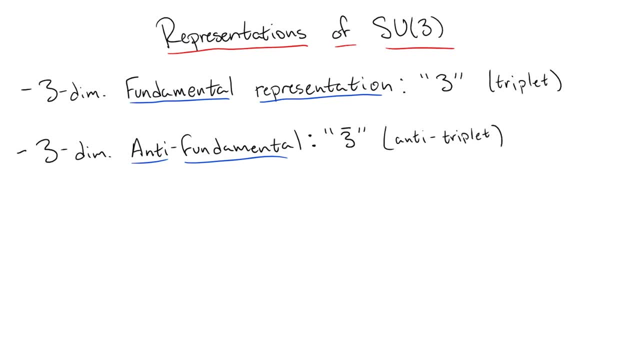 interpreted as the conjugate of the fundamental representation. This is very nice since it has a convenient physical interpretation. The quarks transform in the fundamental representation with red, green and blue quantum numbers, while anti-quarks transform in the anti-fundamental with anti-quark. Now the fundamental representation of the fundamental. 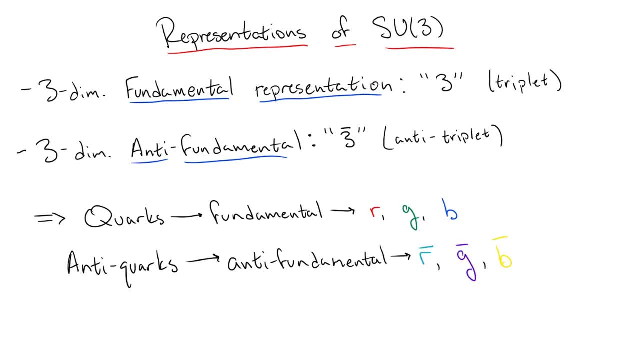 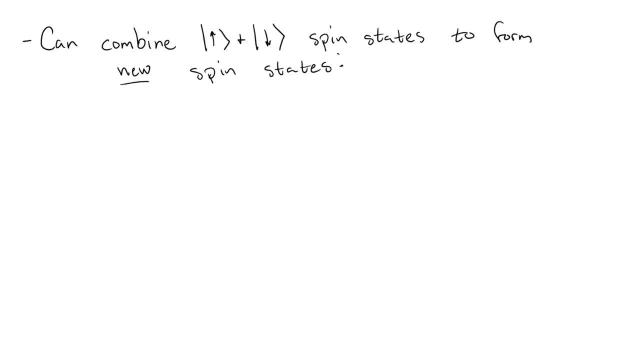 representation is the same as the fundamental representation of the fundamental representation. However, this isn't the end of the story. If we recall, when talking about spin, we were able to combine fundamental spin-half states into different states such as spin0, spin1, and spin3-halves. In fact, these all end up being representations of SU2.. 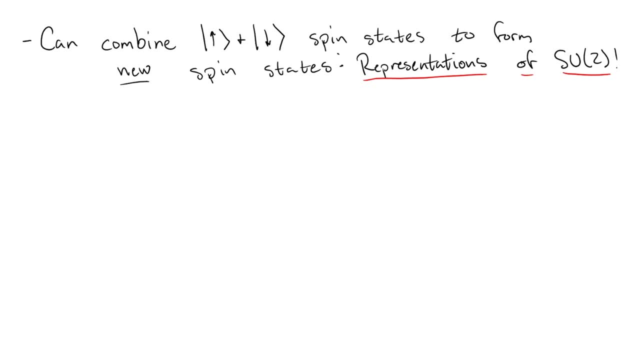 We can combine SU3 fundamental and anti-fundamental states in a nearly identical way to get different SU3 representations, though the actual mathematics of it are a bit more complicated. So, for example, when we combine two spin-one-half particles, we got two states: The spin0 state, also known as the SU2 singlet state, as well as the spin1 state. 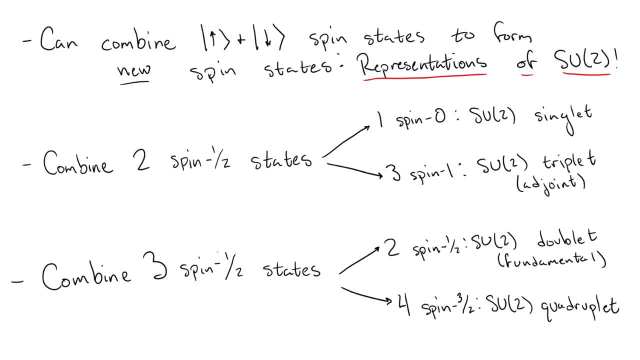 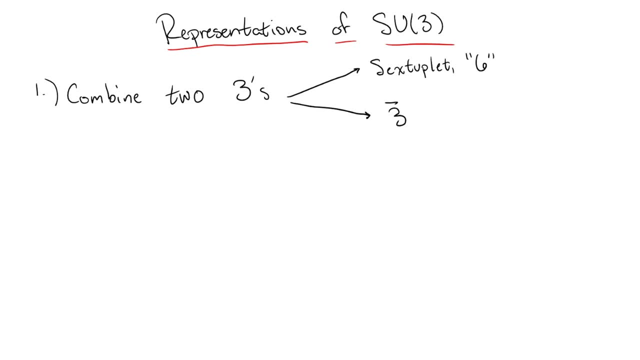 known as the SU2 triplet. Now, when doing the same thing for SU3, we have some options. We can combine two fundamental states, in which case we end up with a sextuplet and an anti-fundamental state. We can also try combining a fundamental and an anti-fundamental, which gives us an SU3 singlet. 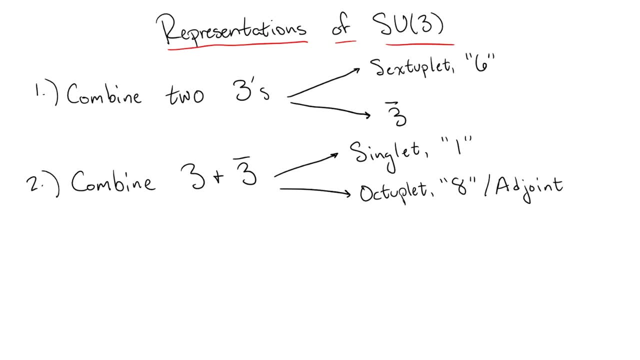 as well as an octet state, which is given the special name of the adjoint representation. Another interesting case is when we combine three fundamentals. This results in a decuplet, an adjoint, a fundamental and a singlet. Now, most of these aren't super important for this discussion. 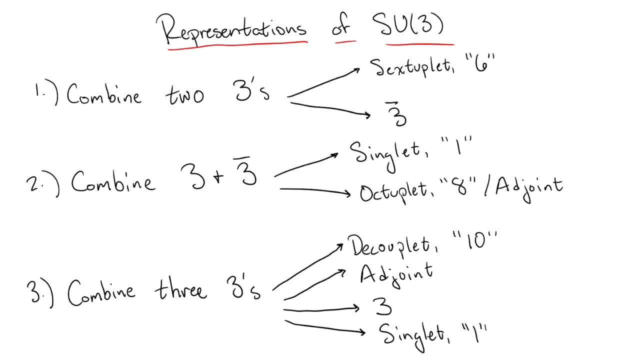 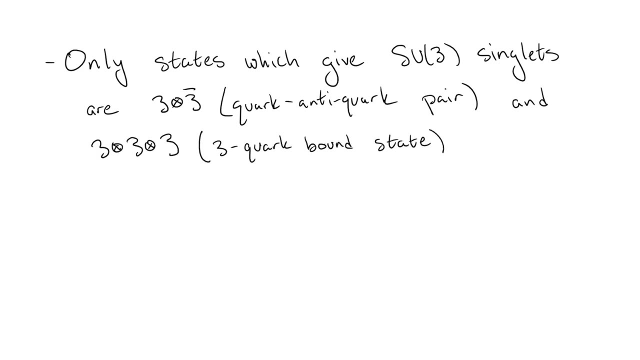 but what is important is the way that we can form SU3 symmetric states, or in other words the SU3 singlets. Notice that in the previous examples, only the combination of a fundamental and anti-fundamental and the combination of three fundamentals gave singlet states. 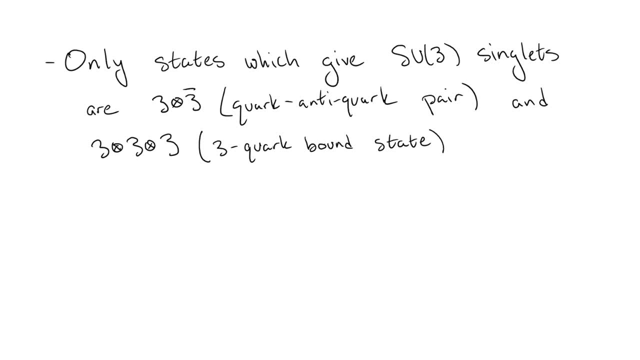 whereas the combination of two fundamentals did not result in a singlet state. If we recall that quarks transform as fundamental SU3 states and anti-quarks transform as anti-fundamentals, we see why we only observe the quark-anti-quark pair, mesons and the three quark baryons. These 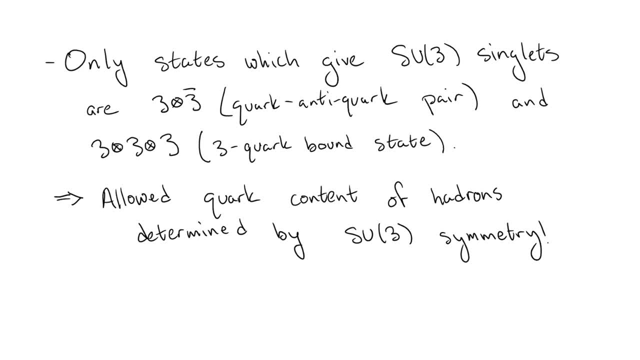 are the only possibilities that are SU3 symmetric. So this explains why we don't observe any quark quark mesons, even though it would seem like they are allowed by isospin. These states are forbidden to be in the situation where nature respects an SU3 color symmetry. 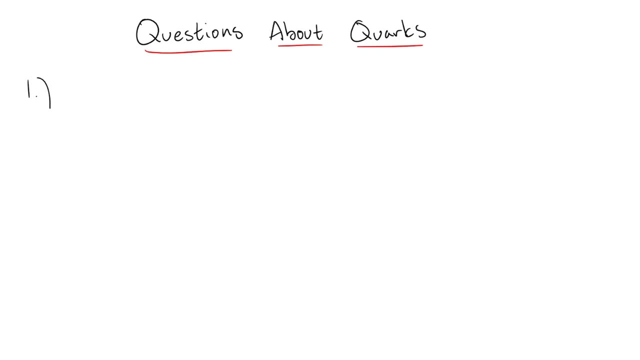 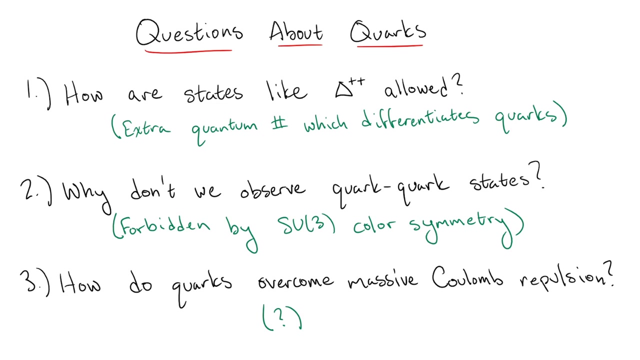 So this extra color symmetry explains a couple of our questions which arose from introducing the quark model. but we still haven't explained how quarks with the same sign electric charge can possibly be bound up into hadrons despite the massive electromagnetic repulsion they feel from. 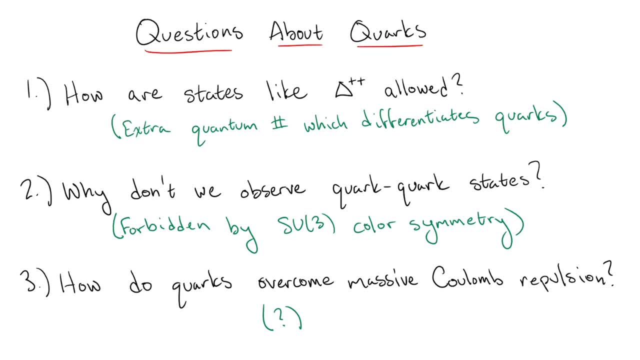 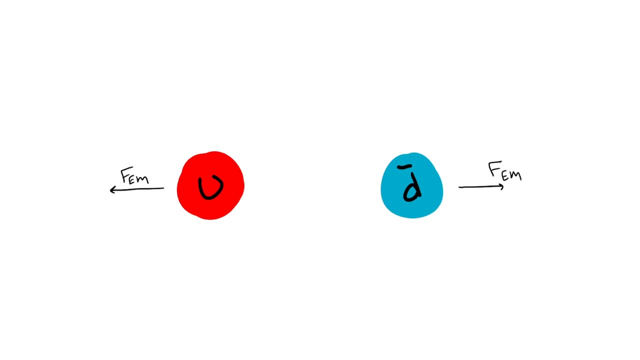 being so close together. The answer to this is actually pretty simple: There must be some other interaction that the quarks feel which competes with electromagnetism to bind the quarks together. This interaction must also be significantly stronger than electromagnetism in order to win. 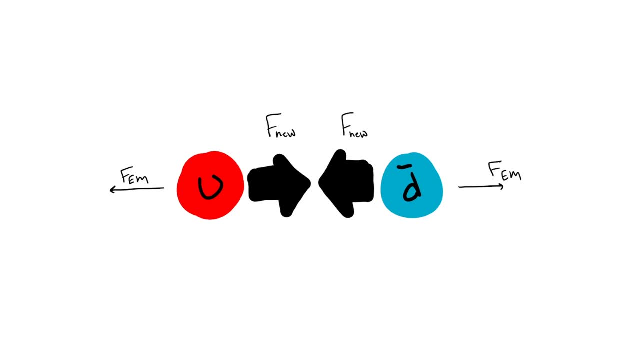 out and keep the hadrons from breaking up. However, there is another subtlety: If there's an interaction which is much stronger than electromagnetism, we don't see it on large length scales. So this new strong interaction shouldn't really lead to a strong interaction. 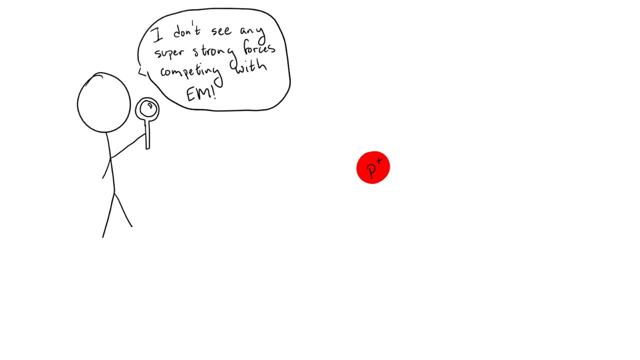 but we could see that the charge would practically leak out of the hadrons. Otherwise we would see it competing with electromagnetism on, say, the molecular level. If there is some charge associated with the interaction, then the hadrons should be neutral. 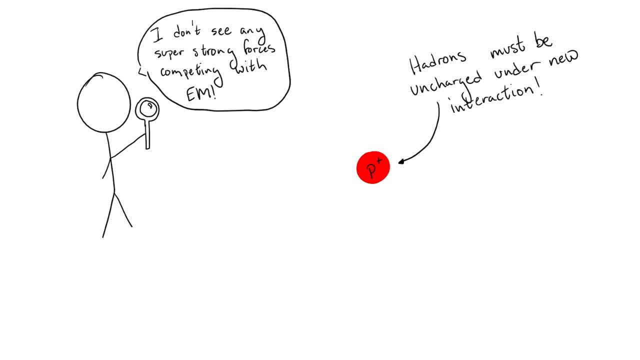 under this charge, Very similar to how atoms, which are bound states of electrically charged particles, when seen far away, are electrically neutral. But we already know of a quantum number, hadrons color. So if we are able to upgrade this color quantum number to a charge under some, 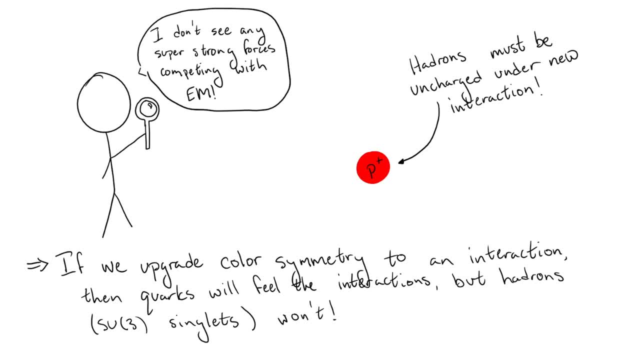 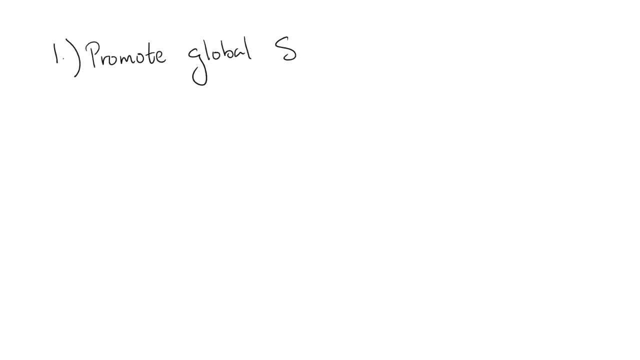 interaction. this would seem very promising, Since we know that our theory is symmetric under SU3 color transformations. we can use the machinery we used to arrive at quantum electrodynamics to turn a symmetry into an interaction, promote the global symmetry to a local one and introduce 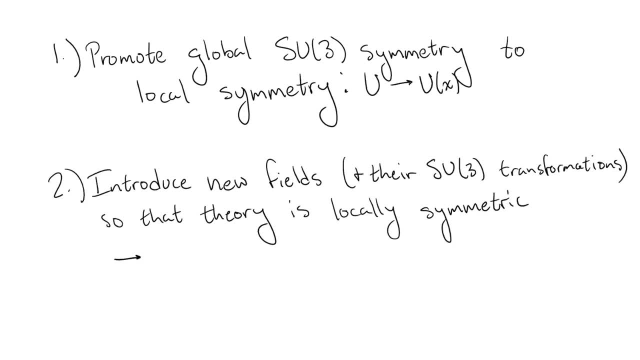 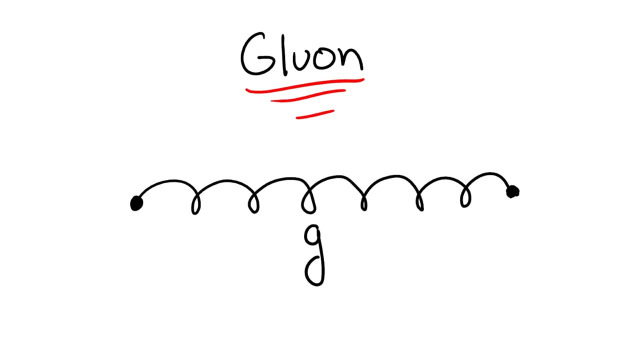 any new fields, as well as any interactions that are necessary to enforce this local symmetry. We can, of course, do this, and we find some interesting results. First, just like the case of QED, we find that we need to include a new field called the gluon in order for the local 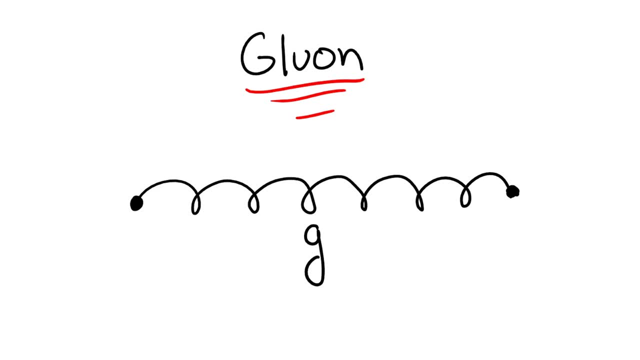 transformations to cancel. in the theory, We can think of these gluons as mediating the color force, in the same way that photons mediate the electromagnetic force. Now, in the case of QED, we can think of these gluons as mediating the color force. 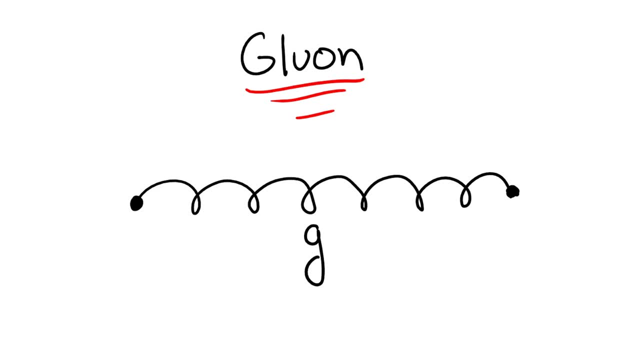 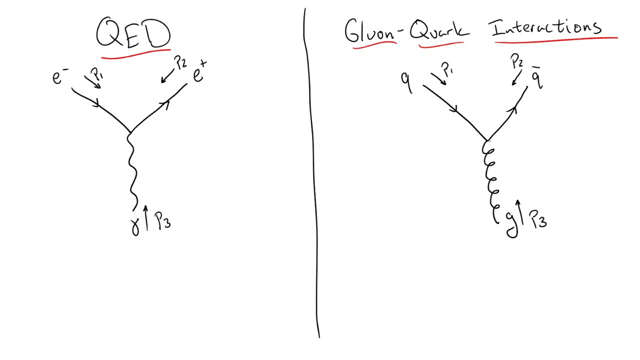 In the language of Feynman diagrams and perturbation theory, the fundamental vertex associated with the interactions between quarks and gluons looks very similar to that from QED, where, if we assign all momenta as incoming, we have a quark, anti-quark and gluon entering. 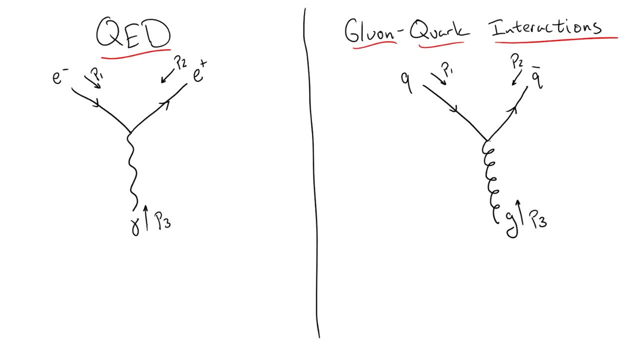 the vertex, whereas in QED we have an electron, positron and photon entering. In the QED case, we see that in order to conserve charge, we need to include a new field called the electron. The photon must be electrically neutral, since the positron and electron have 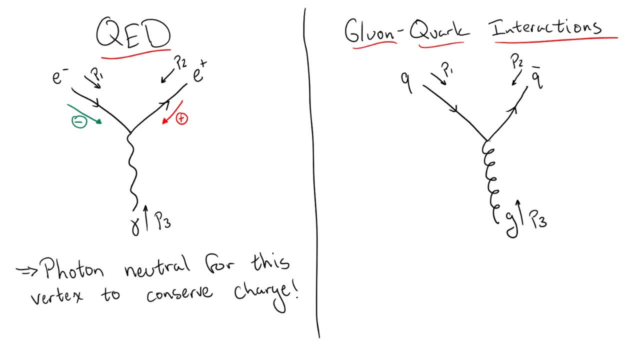 opposite charges. However, for the quarks and anti-quarks, there isn't just a single charge, like we had in QED. There are the three fundamental color charges and their anti-fundamental counterparts. This means that the gluon must be a combination of a fundamental 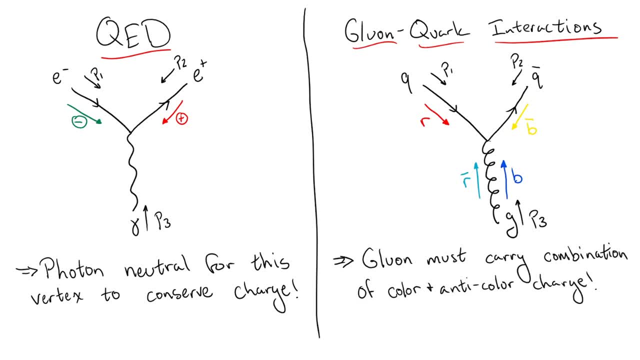 color charge and an anti-fundamental color charge. As we already discussed, when we combine a fundamental and an anti-fundamental SU3 charge, we have two options: an SU3 singlet or an SU3 octet or adjoint. Without getting too deep into the depths of the math, 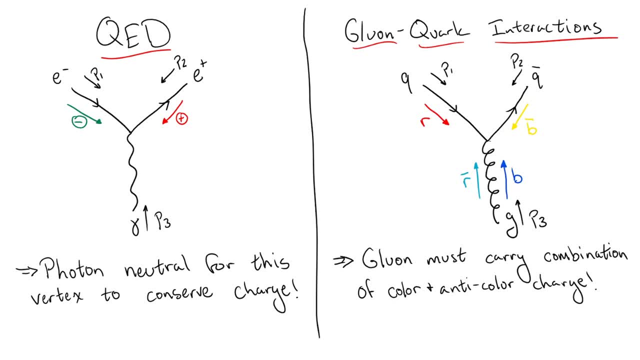 it turns out that the only way to actually preserve the local symmetry is for the gluon to be in the adjoint representation. This can be somewhat seen by the fact that there are eight unique possible SU3 transformations, one transformation for each charge of the gluon. 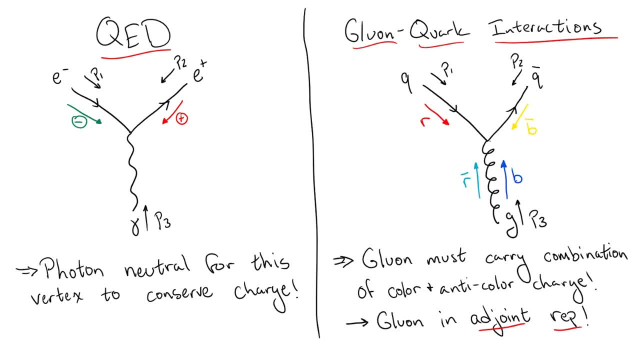 The result is that the gluons themselves carry color charge, though not the red, green and blue of the fundamental representation that the quarks live in. Since gluons also mediate the color force, they must interact with themselves. This is in complete contrast with QED, where photons never 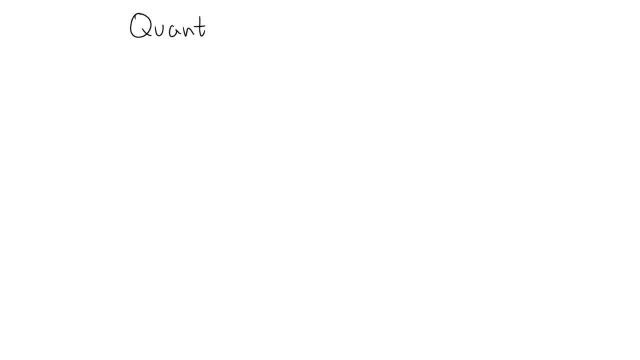 directly interact with each other: The theory of self-interaction. the interactions of the gluons, along with the interactions between quarks and gluons, is known as quantum chromodynamics, or QCD for short. A subtlety here is that, since the gluon 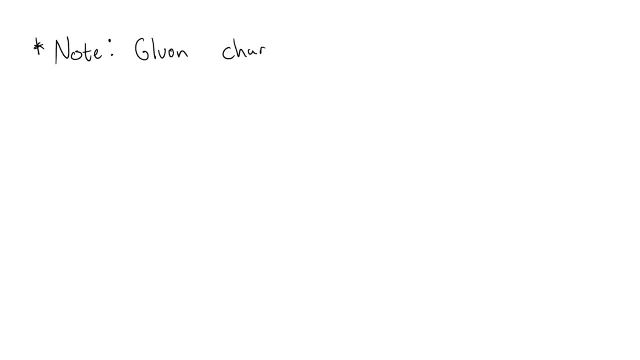 charge is a combination of a fundamental and anti-fundamental charge. when we charge conjugate the state, we still get a combination of a fundamental and anti-fundamental charge. so the gluon ends up still being its own antiparticle, just like the photon. 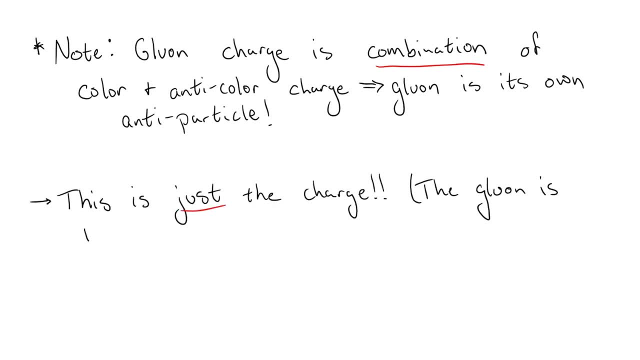 I want to emphasize that when we say the gluon is a combination of a fundamental and anti-fundamental to form an adjoint, this is not the same as saying that the gluon is a quark-anti-quark pair. like the mesons, The gluon is most definitely its own particle, not a composite. The discussion of 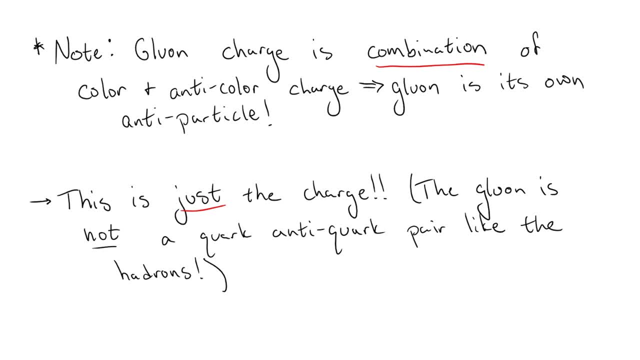 the gluon's charge is about its SU3 transformation properties only, not its internal particle content, because according to QCD it has to be a composite. In other words, it is a component, not a particle. But if I say that the gluon is a combination of a fundamental and anti-fundamental, then the gluon 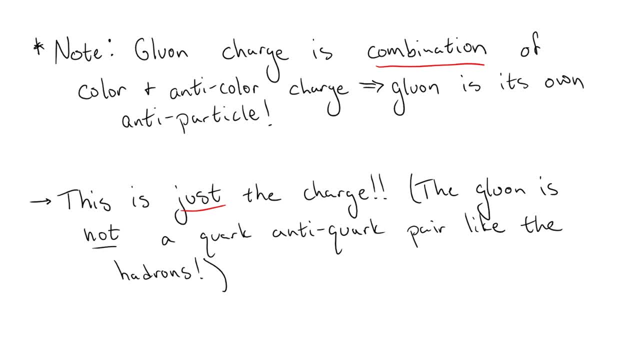 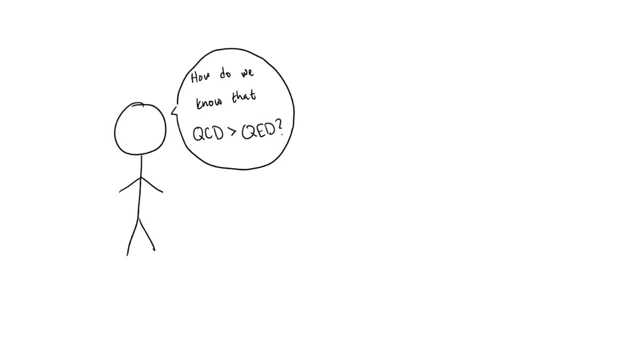 no internal particle content. We've now successfully introduced a new interaction, but how do we know that it's stronger than electromagnetism? The strength of these sorts of interactions is described by a coupling constant, essentially just a number, where the larger it is, the stronger the 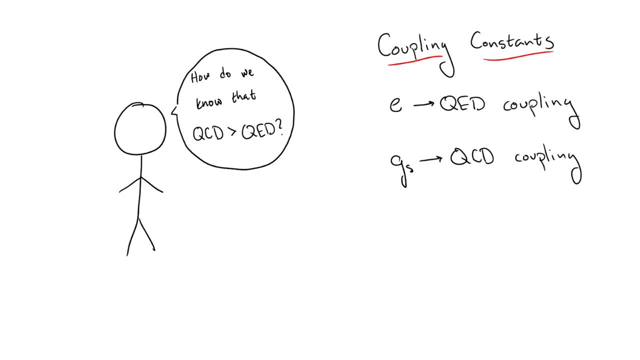 interaction. So we could just say that the QCD coupling is much larger than the QED coupling. constant wash our hands and be done with it. This is easily seen in the leading-order case of a scattering event with an up quark and an. 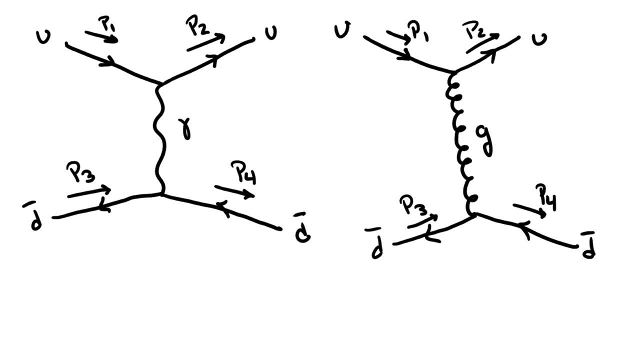 anti-down quark. Both of these particles interact with QED as well as QCD, so if the QCD coupling is much stronger than the QED coupling, then the gluon exchange diagram will have much more influence over the total amplitude than the photon exchange diagram. However, it 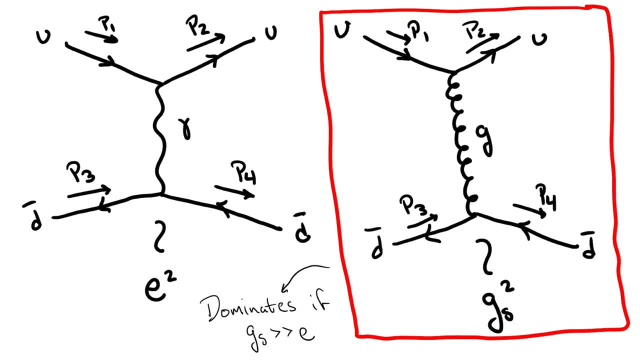 doesn't mean that the QCD coupling is much stronger than the QED coupling. It turns out that there is much more depth to the story than that. In fact, this all comes down to renormalization. Now, if you've seen my video on, 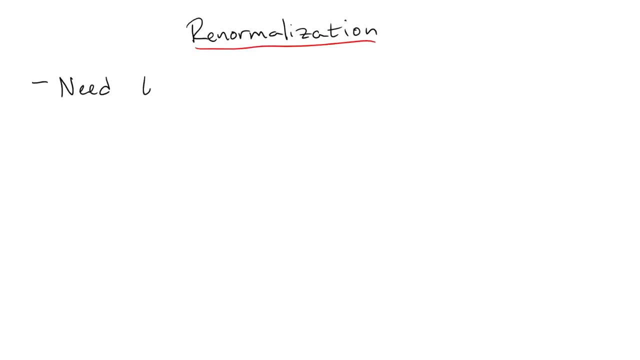 renormalization. you know that these coupling constants must be renormalized to eliminate ultraviolet divergences. They also pick up a quote-unquote artificial energy scale dependence described by the renormalization group equations. Now I say that the scale dependence is artificial because it has 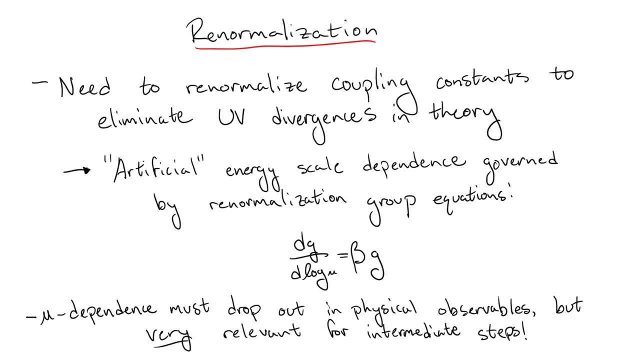 to drop out of the QCD coupling equation, and that's because the QCD coupling has to drop out in the end result whenever we calculate a physical observable. But in intermediate steps this scale dependence can certainly come into play. So what exactly do we find for the scale dependencies of these couplings For QED? 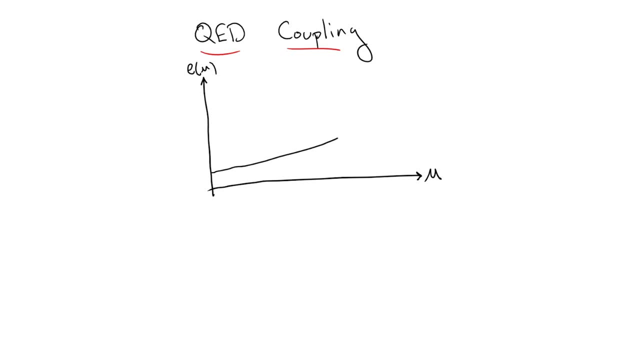 as we increase this energy scale, the strength of the coupling also increases, Since in particle physics terms, higher energies correspond to shorter length scales. we can also say that the electromagnetic coupling gets stronger the closer two charged particles are to one another. Note that this is not the same. 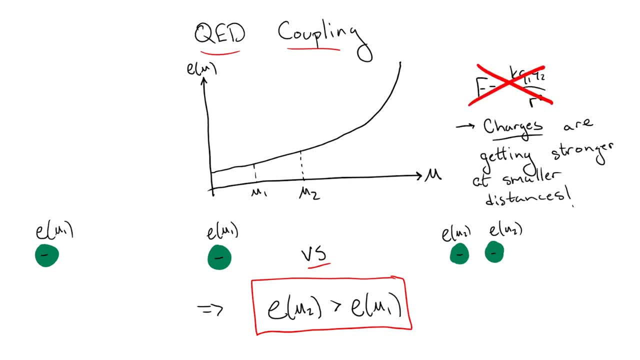 thing as the inverse square law from electromagnetism. This is essentially saying that the charge of the electron gets larger as it gets closer to another electron, for example. This can also be rephrased in terms of quantum screening effects and vacuum polarization, but this isn't really the point of this video. 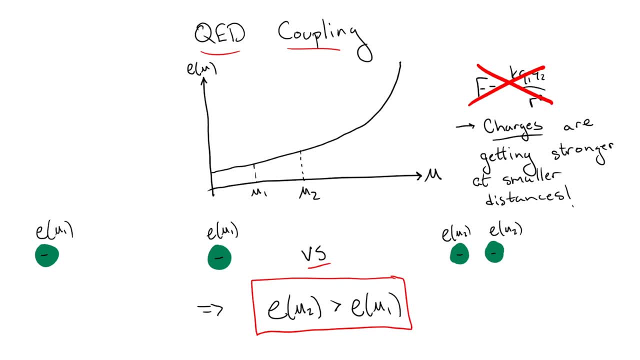 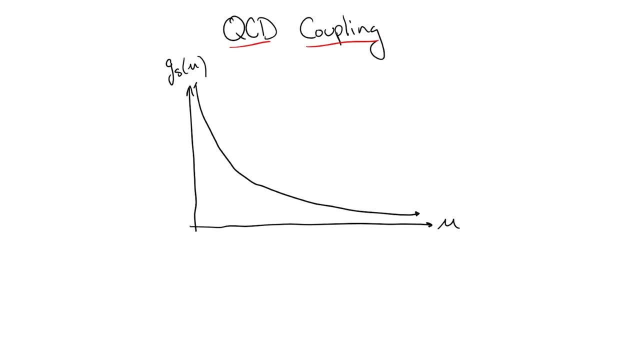 What about for QCD? Well, it turns out that gluon self-interaction, which is a very common phenomenon, introduces an interesting effect, Namely that as long as we don't have too many quarks in our theory, the QCD couplings get stronger at lower energy scales, a phenomenon 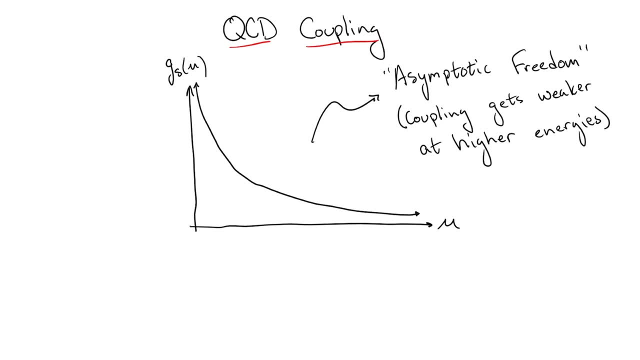 known as asymptotic freedom. In fact we find that in any feasible particle physics experiments the QCD effects must almost always dominate. Another consequence comes from considering perturbation theory. We know that we typically do perturbation theory in powers of couplings, So when the couplings get large perturbation, 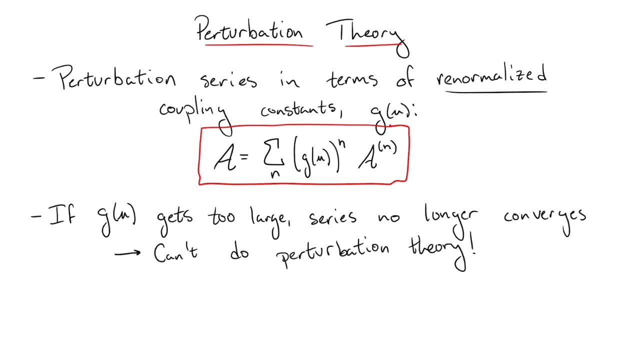 theory will completely break down, since this sort of power series no longer converges. For QED, this isn't a huge deal, since it doesn't become non-perturbative until insanely high energies, much larger than the Planck scale. However, since the QCD coupling gets large at 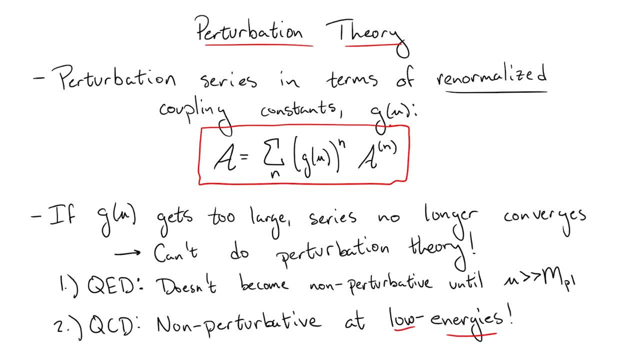 low energies. QCD is completely non-perturbative at low energy scales and we can't use our typical Feynman diagram expansions or any assumptions that we can treat the external states as free single particle states. This means that it doesn't really. 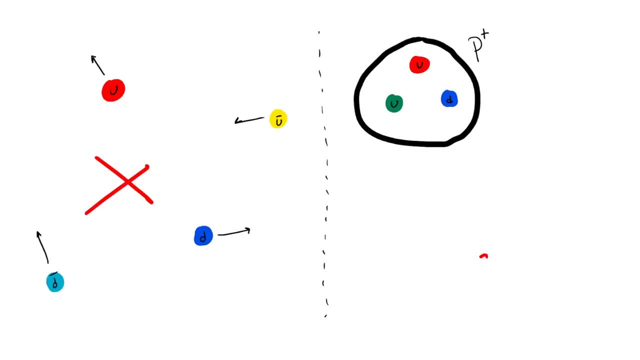 make sense to talk about a free quark in this regime. We should expect them to always live in bound states, But this is exactly what we observe: The quarks always bind together to form hadrons. So let's recap what QCD does for us. The color charge gives us an extra. 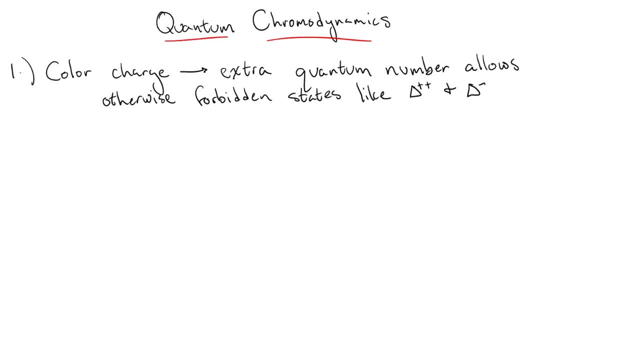 quantum number to play with in order to allow seemingly forbidden combinations of quarks like the delta plus plus and delta minus baryons. The fact that QCD arises from an SU symmetry means that the bound states formed from quarks should be colorless SU singlet states, which disallows